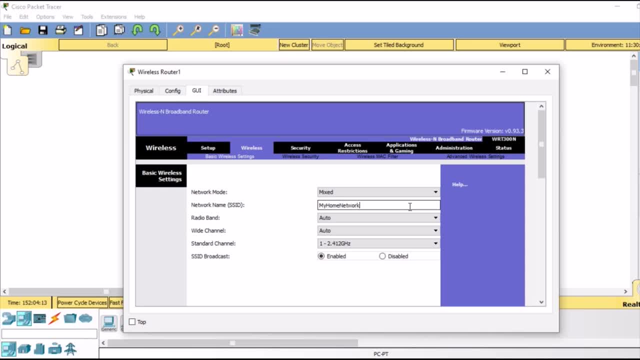 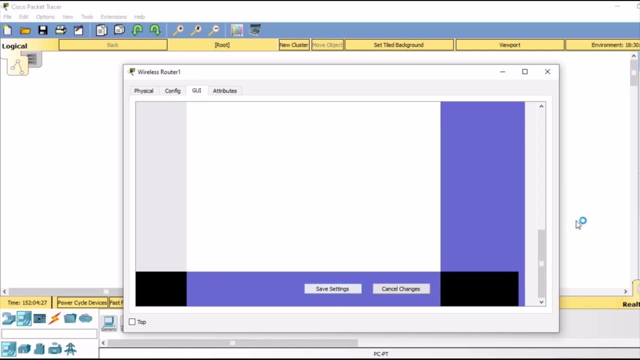 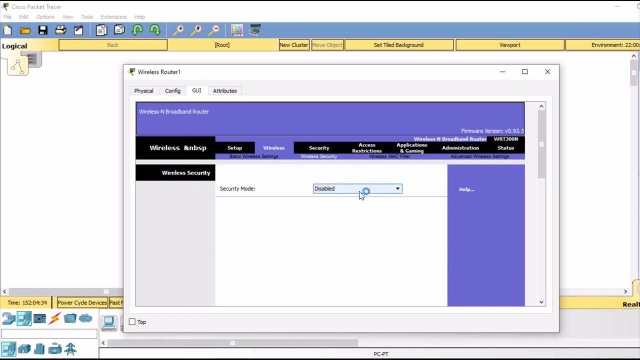 To my home network and the remaining settings. that would remain the same, and the standard channel and all other options, and we are going to go to the bottom and going to save these settings, Save settings. and then, finally, we are going to enable security In wireless security. we are going to select a security mode and that would be WEP web. This is a security protocol. 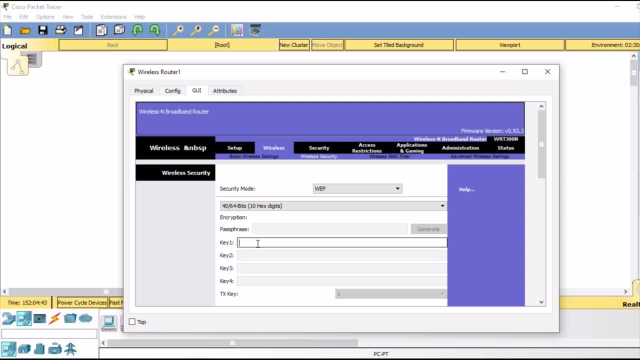 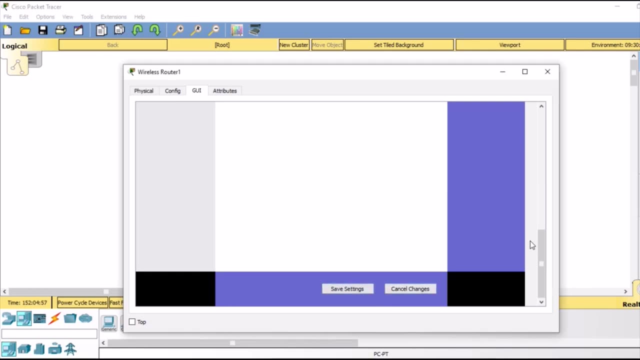 And we are going to give it a security key, 01234567, and then we are going to save it Again at the bottom, save settings, But here it is giving us the error. We have to increase the number of digits for the security code. So we are going to give the key 0123456789. 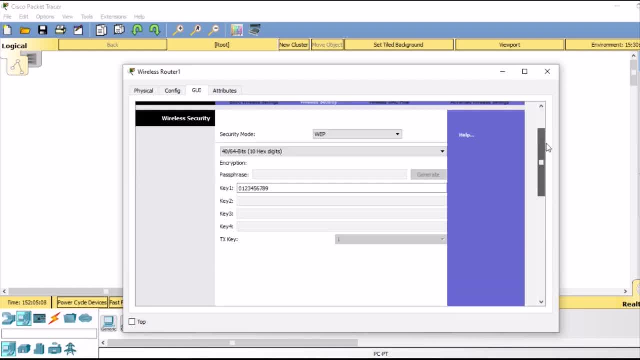 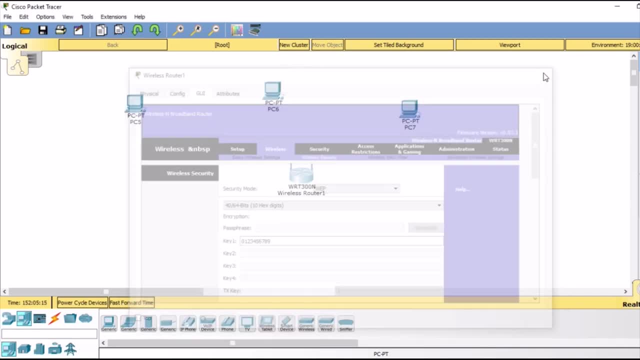 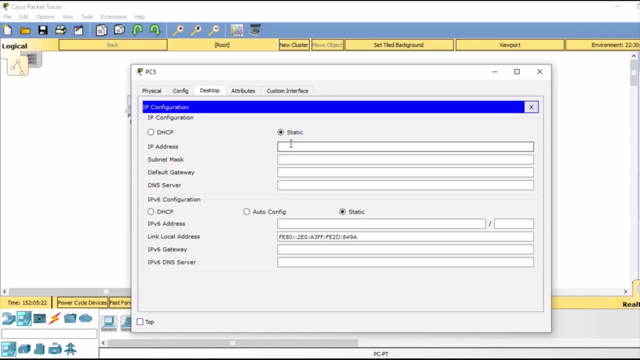 Finally, we are going to save these settings and we are all done with our wireless. So after that, we are going to close this router and we are going to give our PCs static IP addresses. Double click the PC, Then in desktop, go to IP configuration. I am going to give it an IP address of 192.168.0.5.. And then we are going to give default gateway 192.168.0.1.. This is the IP address of our wireless router. 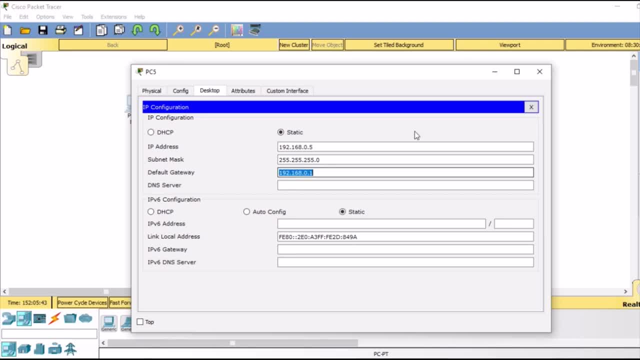 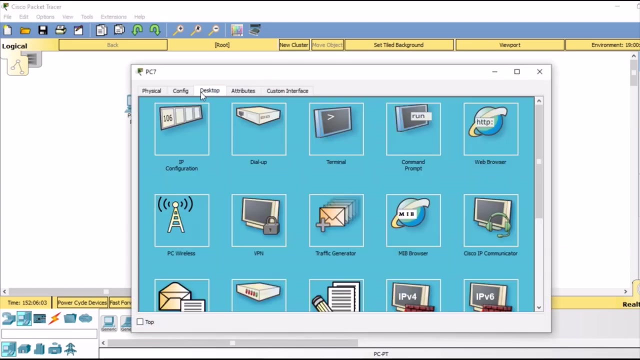 Because we want to connect our PC with that router. So we are going to give this IP address of our wireless router. Similarly, we are going to the next PC desktop IP configuration. We will give it IP address of 192.168.0.6.. Then, similarly, the same default gateway of our wireless router. Finally, our third PC desktop IP configuration: 192.168.0.7.. Here we are going to give our IP address of 192.168.0.7.. And then we are going to give our wireless router. 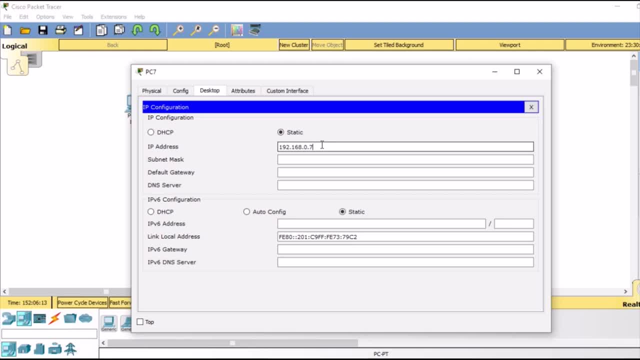 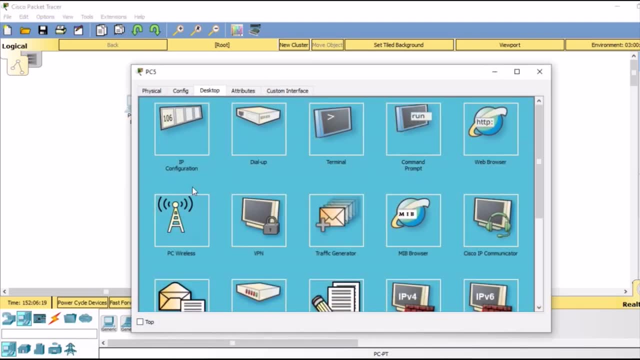 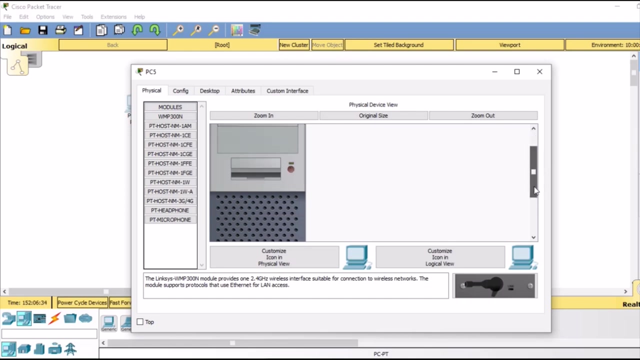 We are going to give the IP address to our third and last PC And the default gateway of our wireless router. So we are again going to double click and we are going to go to PC wireless. Here the interface of wireless is missing on the PC. So we are going back to the physical tab of this PC And we are going to turn off the PC by clicking this red button. Then we are going to go to the bottom and we don't have any place to add a new interface, So we will delete this. 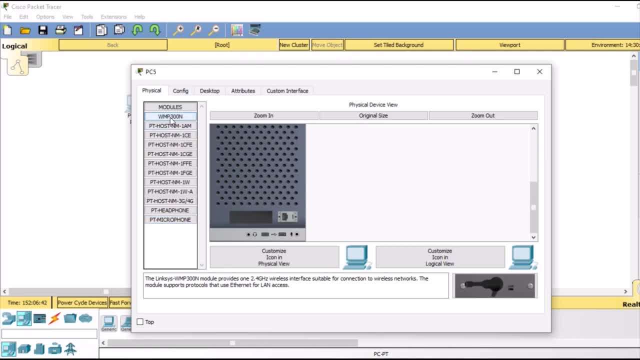 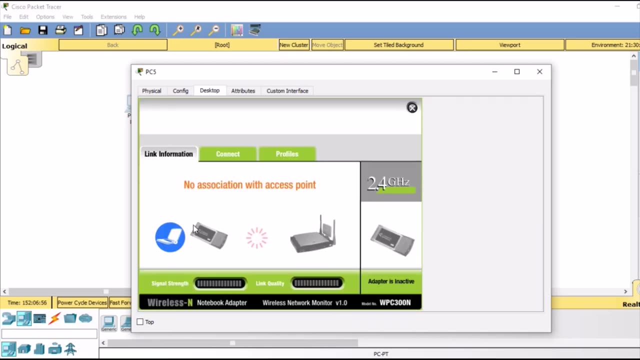 By dragging it back, Selecting WMP300N and dragging it to the place where we deleted the previous interface. So we are going to again turn on our PC. Then we are going to go to the desktop In desktop PC wireless Here, But it's not connected to the access point. We are now going to go to the connect tab And we are going to click wireless mode And here you are going to click connect And you have to give the key. 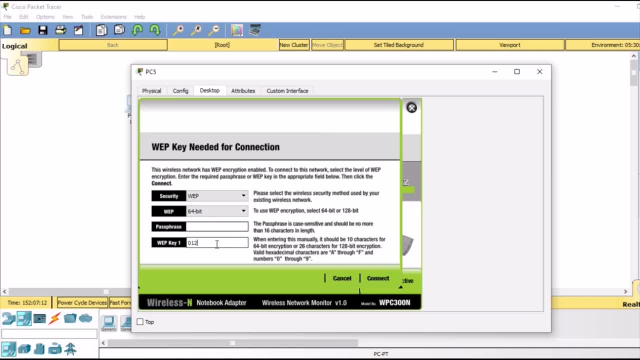 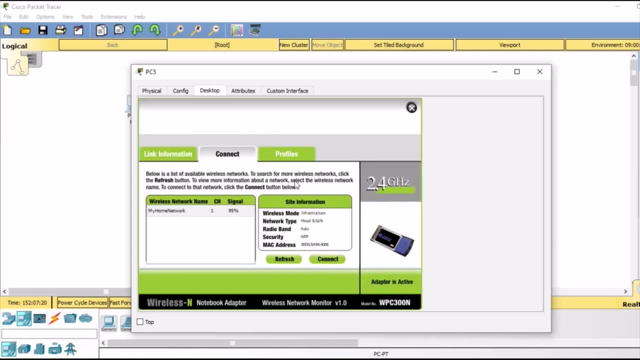 WEP Web Key 1. Which was from 0 to 9.. So we are going to give the key And then we are going to click connect And in the link information, when we click that Here, you can see we have successfully connected to our access point. 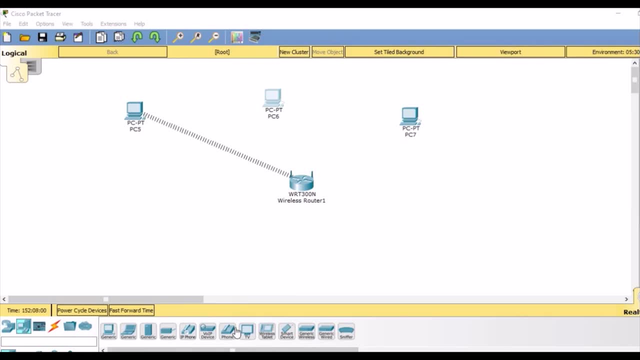 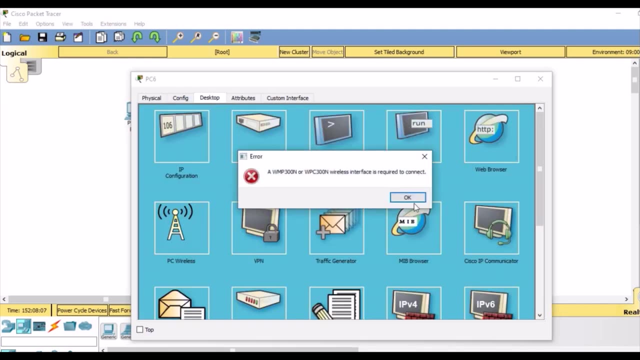 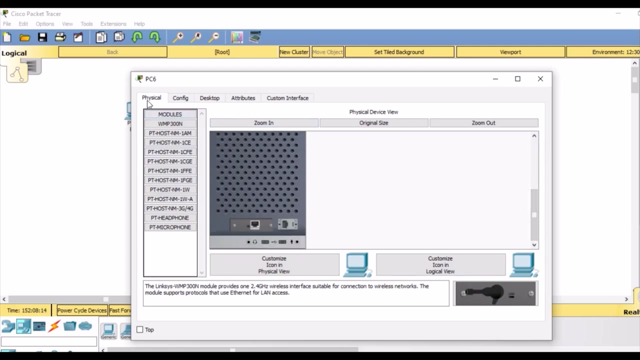 Similarly for the next PC, PC number 2.. We are simply going to double click it And we are going to go physical connection First, PC wireless. It does not have the required interface turn it off. we are going to drag back this interface that is already there to. 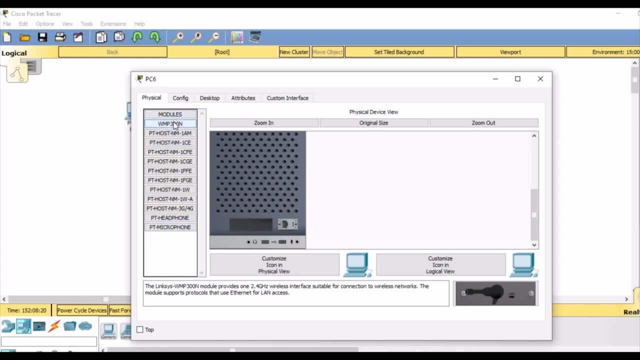 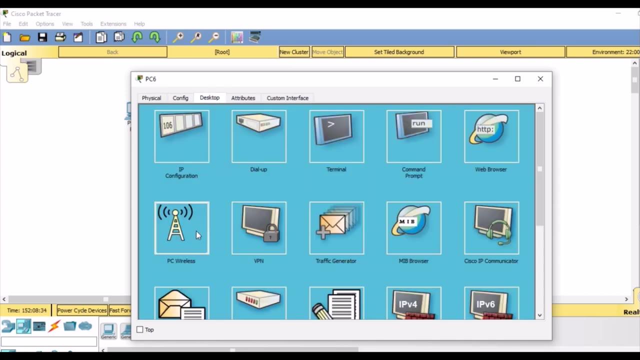 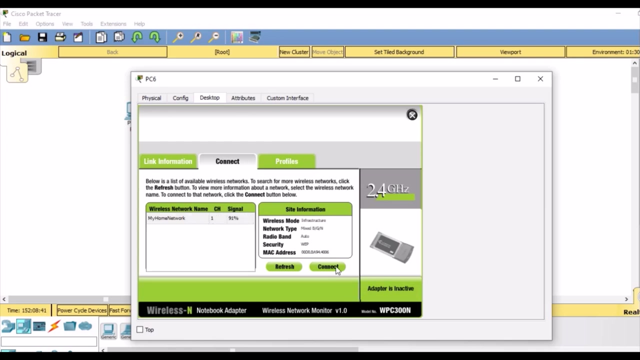 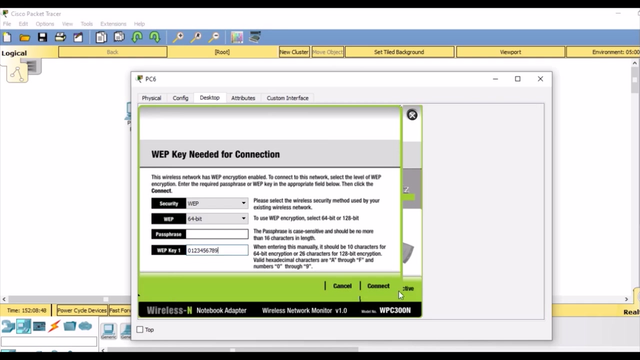 delete it or remove it. then click WMP 300 in and place it where we had our previous interface. so carefully. drag and drop it. then turn it on. and now go to desktop PC Wireless- no connection- connect wireless mode. we are going to give our key- that was from 0 to 9, the web key: 1, 0, 1, 2, 3, 4, 5, 6, 7, 8, 9, connect. 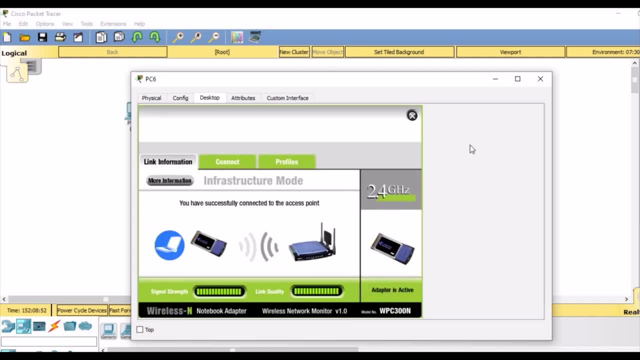 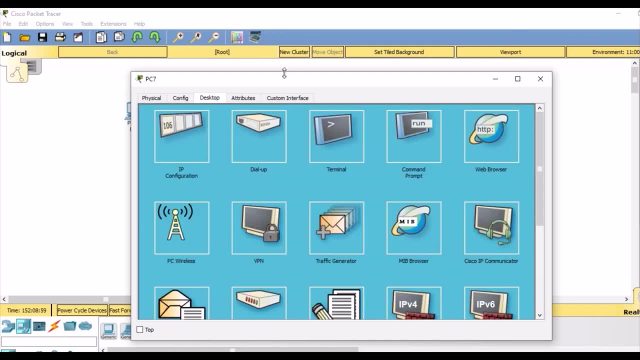 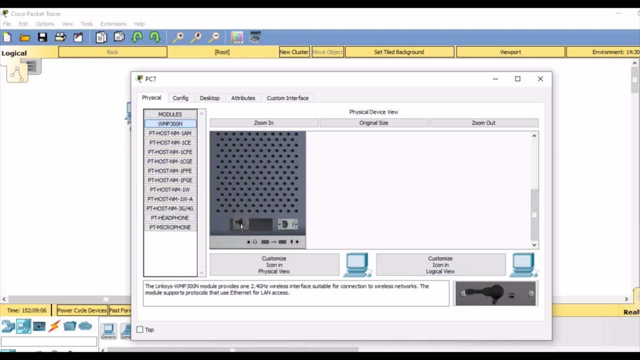 similarly and go to link information. now we have successfully connected, finally, our third and last PC. similarly, we are going to connect it, we are going to add the interface by going to the physical tab and again, this WMP 300 interface would be added to enable wireless network. 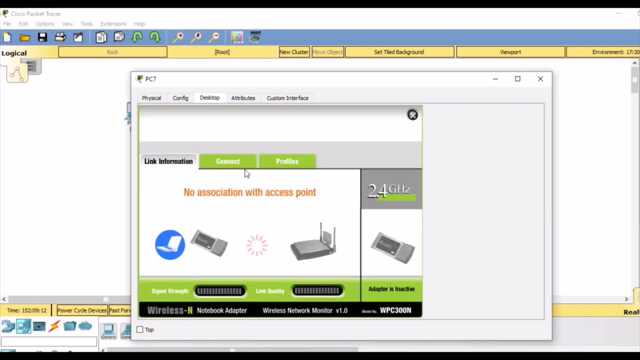 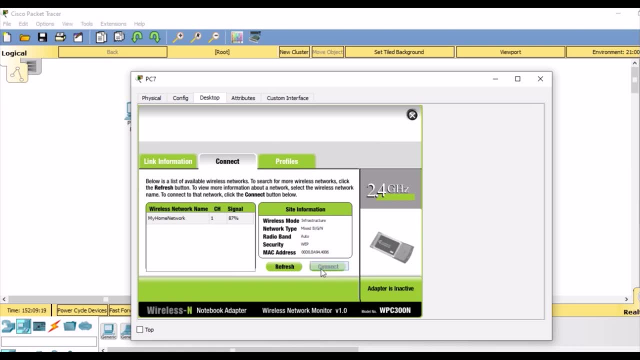 okay, let's go to desktop again: PC Wireless- the same steps: connect and giving it the correct key that we configured for our wireless LAN, for the router, the wireless router. we are going to connect it and link information and it is now connected and you can already see these wireless connection among.